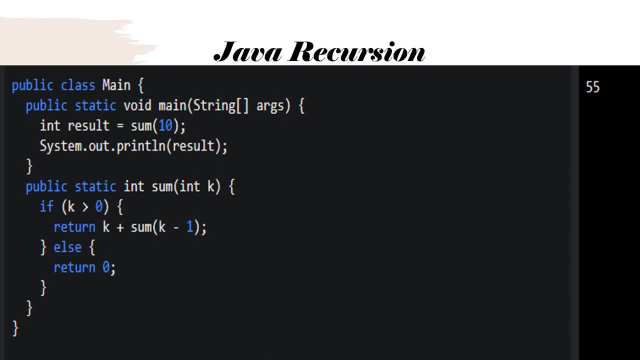 At this point, the function returns zero and the cumulative sum is returned to the caller. 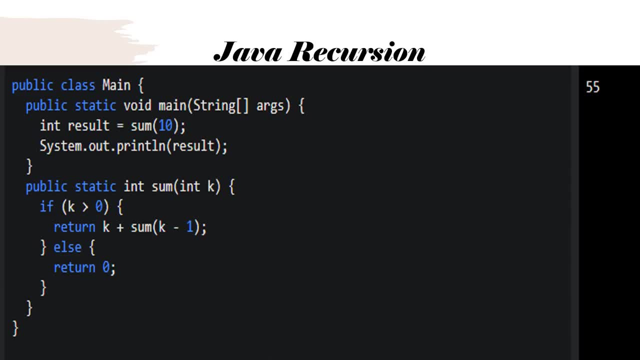 The function calls form a chain, with each call building upon the result of the previous call until the final result is obtained. 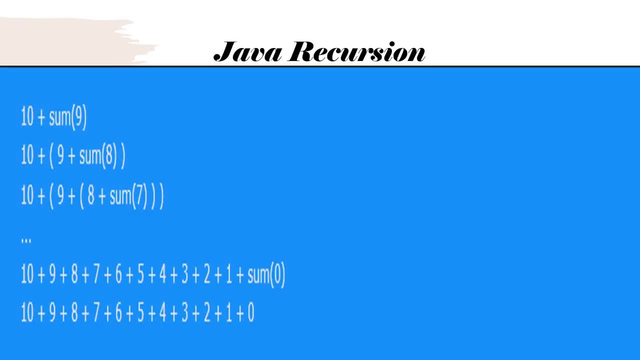 Example explained, when the sum function is called, it adds parameter k to the sum of all numbers smaller than k and returns the result. 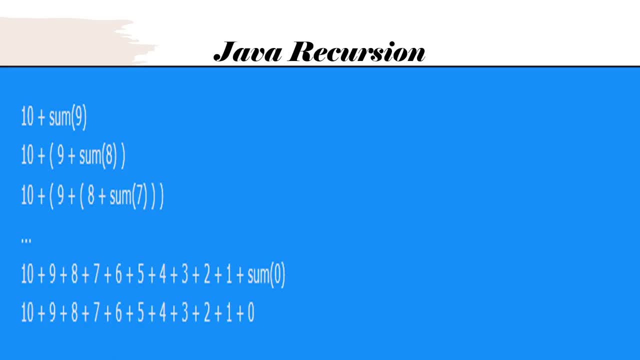 When k becomes zero, the function just returns zero. When running, the program follows these steps. Since the function does not call itself when k is zero, the program stops there and returns the result. 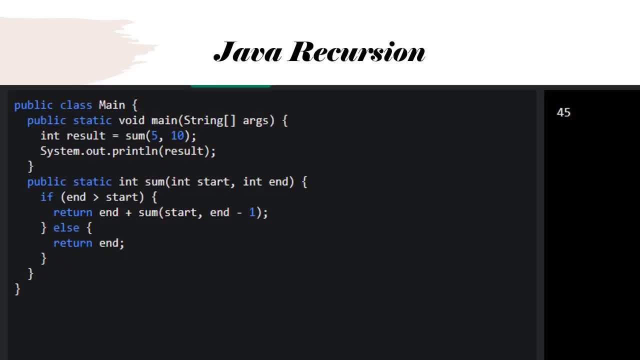 Halting condition, just as loops can run into the problem of infinite looping, recursive functions can run into the problem of infinite recursion. 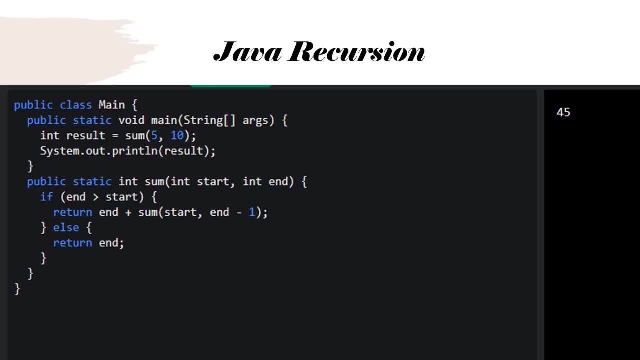 Infinite recursion is when the function never stops calling itself. Every recursive function should have a halting condition, which is the condition where the function stops calling itself. 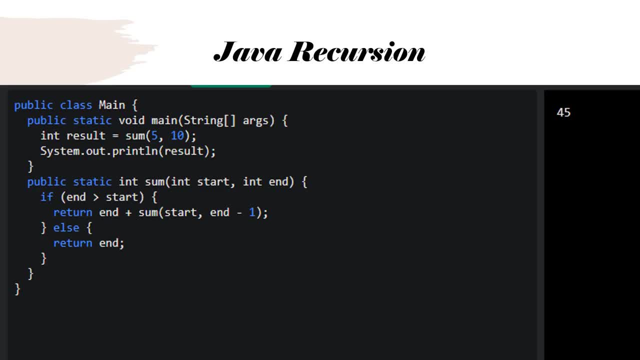 In the previous example, the halting condition is when the parameter k becomes zero. 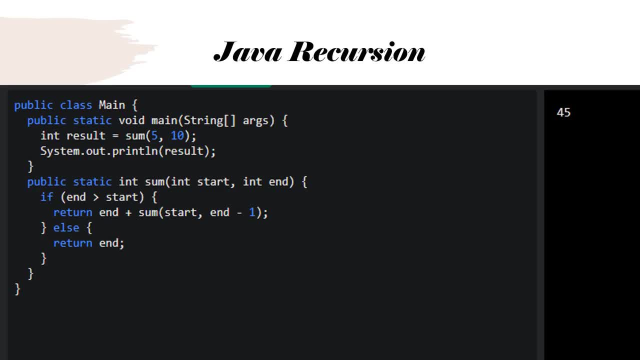 It is helpful to see a variety of different examples to better understand the concept. 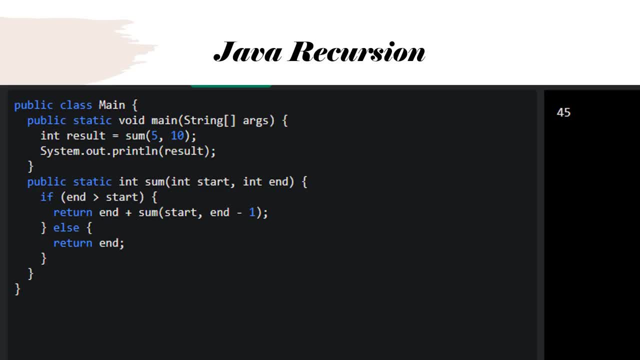 In this example, the function adds a range of numbers between a start and an end. 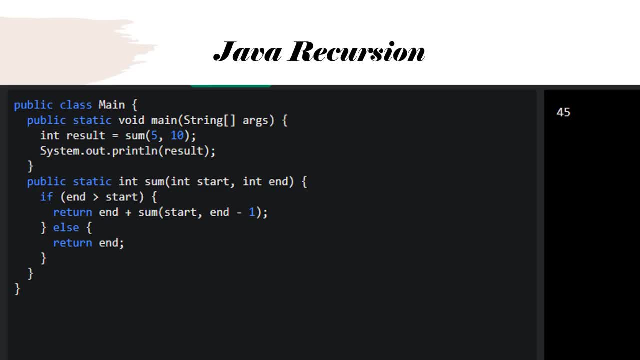 The halting condition for this recursive function is when end is not greater than start. 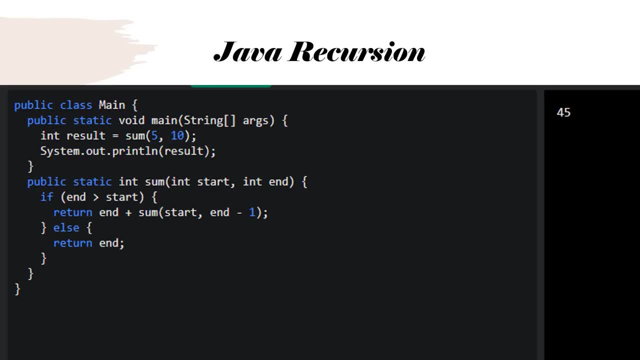 The program is a recursive function, which is a Java code that implements a recursive function to calculate the sum of the numbers from a given start integer to an end integer. 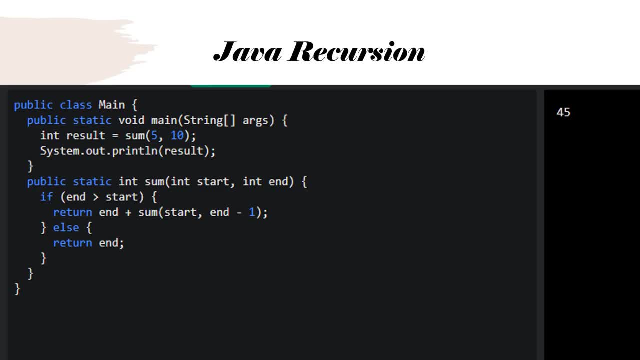 The expected output of the program is the sum of the numbers from 5 to 10, which is 45. 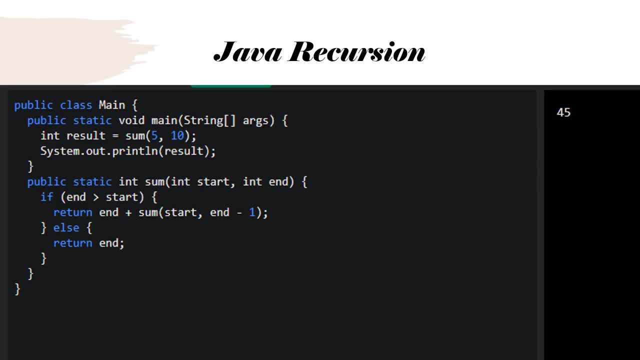 This program implements a recursive function to calculate the sum of the numbers from a given start integer to an end integer. 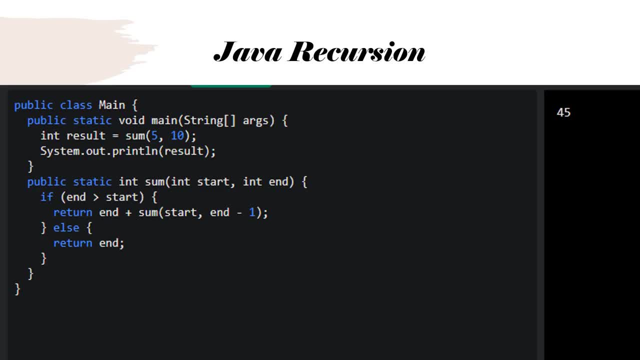 The sum function uses a halting condition to determine when to stop the recursion and return the result. The halting condition is the change in the result. The halting condition is the check if end start, 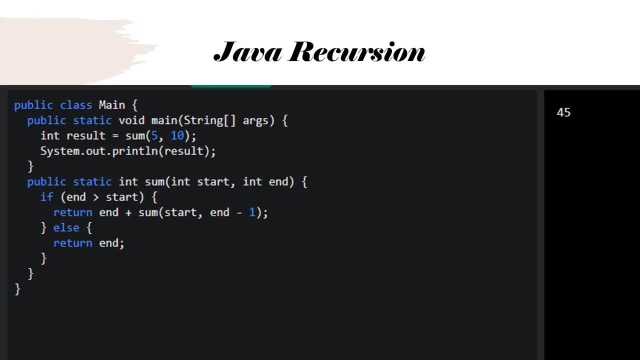 which is evaluated at the start of the function. If the end integer is greater than the start integer, the function returns the current value of end plus the result of calling the sum function with start and end 1. This process continues until end is no longer greater than start, at which point the function returns the current value of end, which is the final result of the sum. 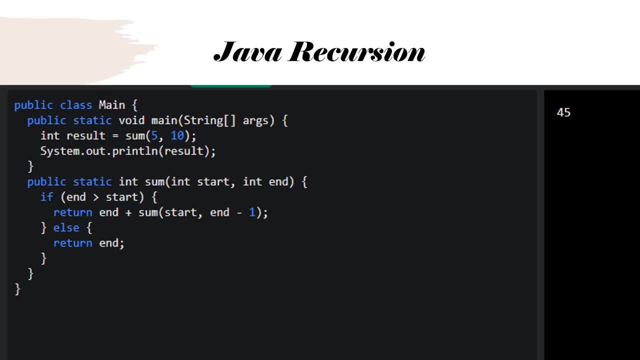 The halting condition is an essential part of any recursive function. As it determines when the recursion should stop. 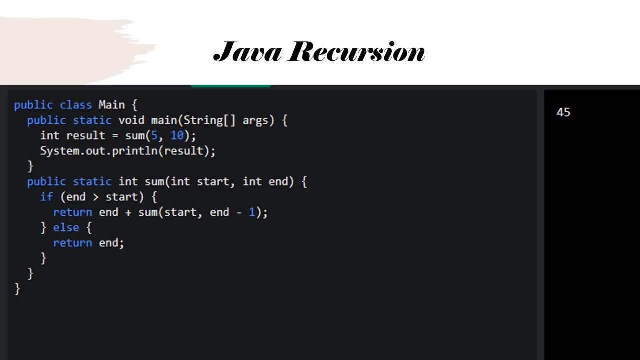 Without a proper halting condition, the function will continue to call itself indefinitely, leading to an infinite loop and a stack overflow error. 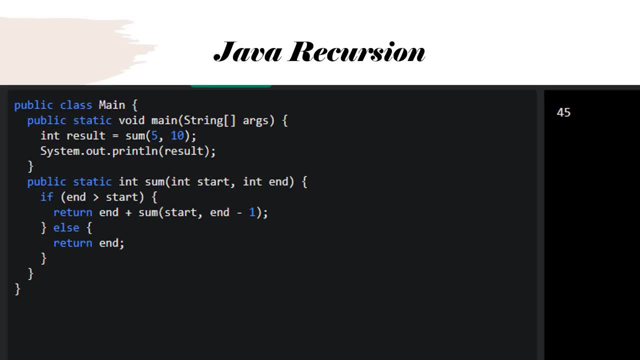 In this program, the halting condition is met when end becomes less than or equal to start, at which point the function returns end, thus terminating the recursion and returning the final result. 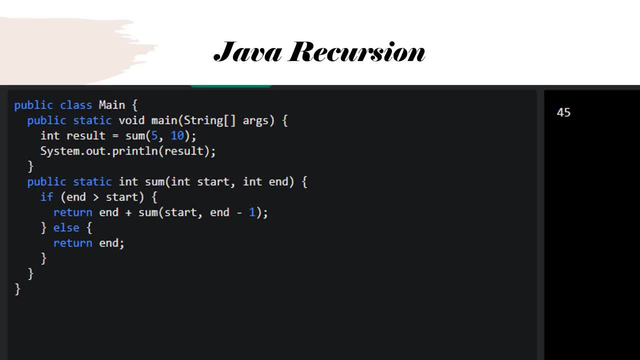 The developer should be very careful with recursion, as it can be quite easy to get lost. It can be quite easy to slip into writing a function which never terminates, or one that uses excess amounts of memory or processor power. However, when written correctly, recursion can be a very efficient and mathematically elegant approach to programming. Encapsulation. 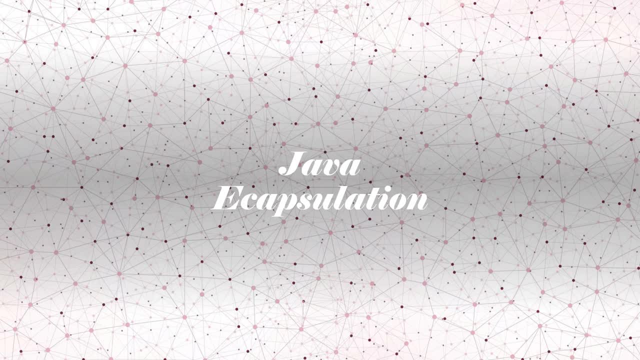 The meaning of encapsulation is to make sure that sensitive data is hidden from users. 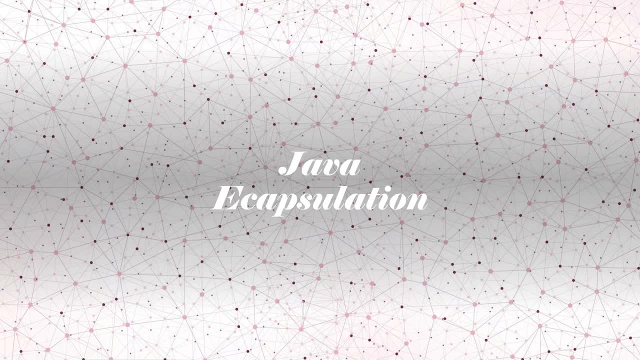 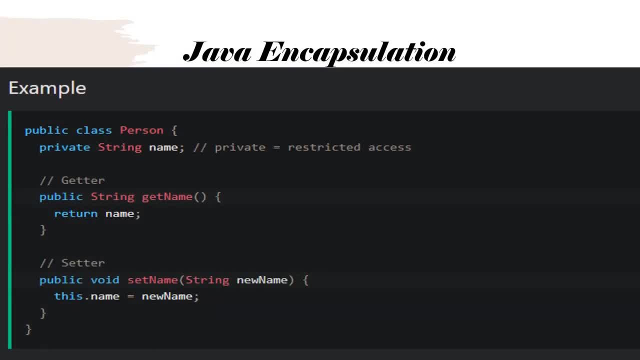 Updating incarnate actions supports our machine to drink small amounts of data once every security невalyzed. Providing that Rep� class does not create very big valores and there are no mass values. 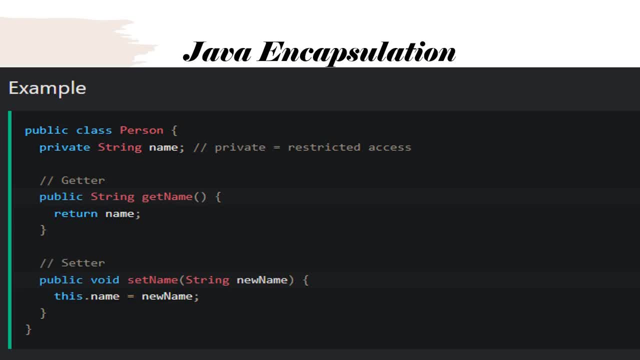 In fact, it should be activate them inıyoruzin's code when UsedValue. However, it is possible to access them if we provide public get and set methods. for both is that they start with either get or set followed by the name of the variable with the first letter in uppercase the program is a java code that defines a class called person with two methods a get name method and a set name method there is no expected output for this program as it is a class definition and not a complete program the methods defined in the class can be used in other parts of the program to retrieve or modify the value of the name field but there is no direct output from the code as written get and set in java are part of the concept of encapsulation which is one of the four pillars of object-oriented programming encapsulation is the technique of making the fields of a class private and providing access to them through public methods the get name method is a getter method as it retrieves the value of the private name field and shown on the left side of the level of the java code that does maintain all the code field. The setName method is a setter method as it sets the value of the private name field. 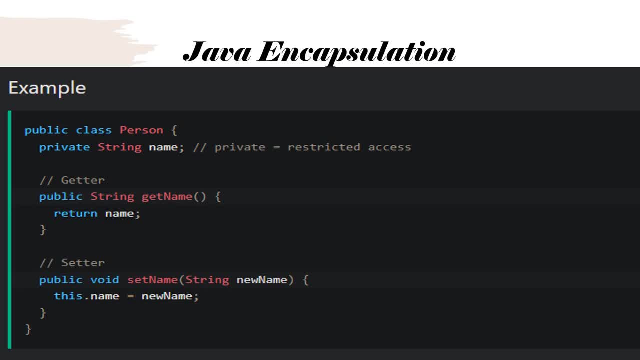 By using getters and setters, the implementation details of the person class are hidden and only the necessary information is exposed to other parts of the program, improving the security and maintainability of the code. Example explained, the get method returns the value of the variable name. The set method takes a parameter newName and assigns it to the 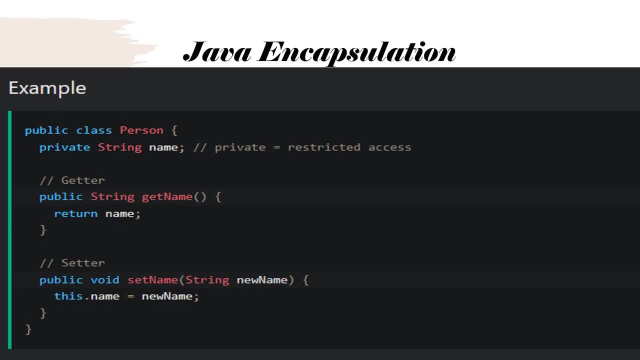 name variable. The this keyword is used to refer to the current object. 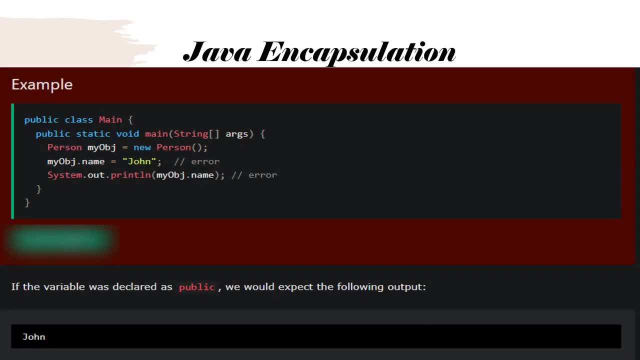 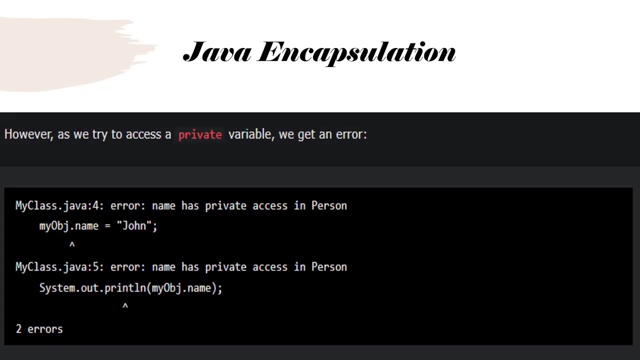 However, as the name variable is declared as private, we cannot access it from outside this class. If the variable was declared as public, we would expect the following output. However, as we try to access a private variable, we get an error. Instead, we use the get name and set name. 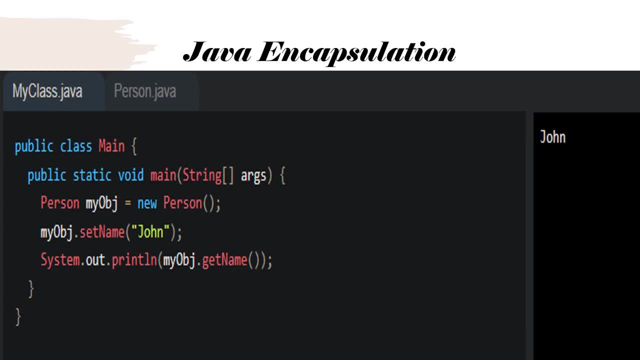 Methods to access and update the variable. The program is a Java code that creates an instance of the person class, sets its name using the setName method, and retrieves its name using the getName method. The expected output of the program is John encapsulation in Java works by wrapping the data fields and behavior methods of an object within a single entity class and providing access to the data only through the methods of the class. In this program, the fields of the person class are declared as private, meaning they can only be accessed within the class itself. To allow other parts of the program to access and modify the name field, the setName and getName methods are provided. The setName method sets the value of the name field, while the getName method retrieves the value of the name field. By accessing the name field only through these methods, the implementation details of the person class are hidden, and the code is more secure and easier to maintain. 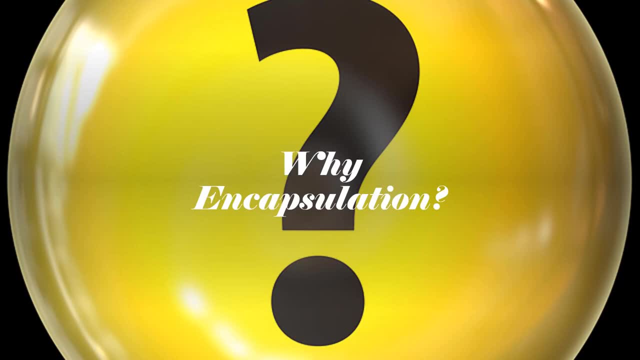 Why encapsulation? Better control of class attributes and methods. Class attributes can be made read-only, if you only use the get method, or write-only, if you only use the set method. Flexible. The programmer can change one part of the code without affecting other parts. Increased security of data. 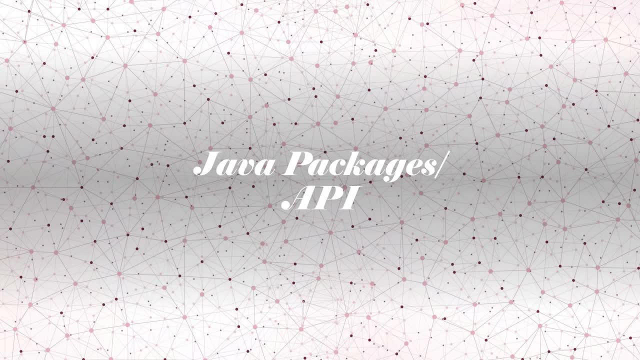 Java Packages API. Java Packages API. A package in Java is used to group related classes. Think of it as a folder in a file 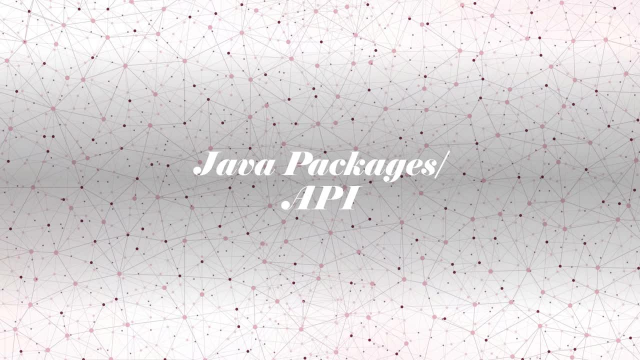 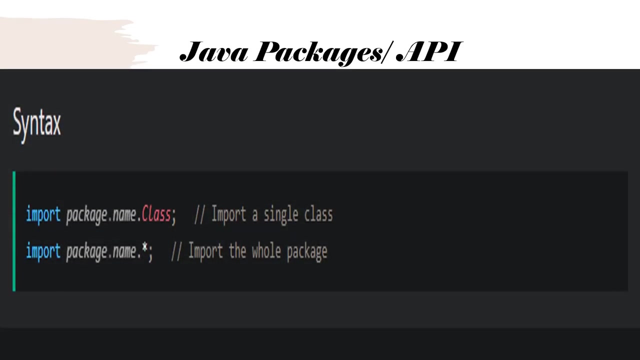 directory. We use packages to avoid name conflicts, and to write a better maintainable code. Packages are divided into two categories, built-in packages, packages from the Java API, user-defined packages, create your own packages. Built-in packages, the Java API is a library of pre-written classes, that are free to use, included in the Java development environment. The library contains components for managing input, database programming, and much, much more. 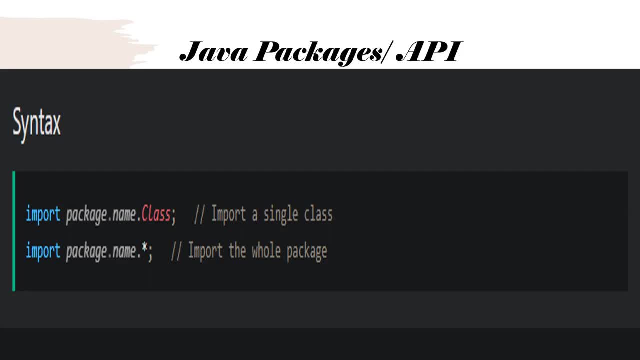 The complete list can be found at Oracle's website, https colon double forward slash docs dot oracle dot com forward slash javase forward slash eight forward slash docs forward slash API. The library is divided into packages and classes. 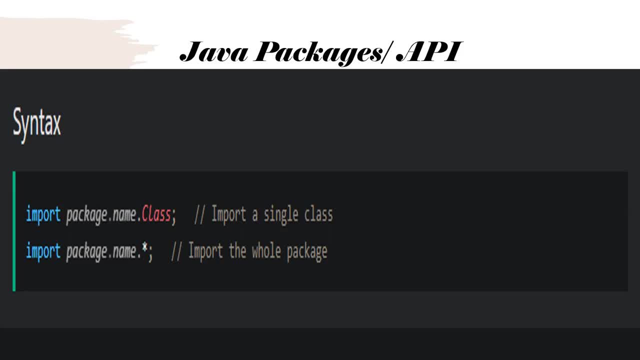 Meaning you can either import a single class, along with its methods and attributes, or a whole package that contain all the classes that belong to the specified package. To use a class, or a package from the library, you need to use the import keyword. 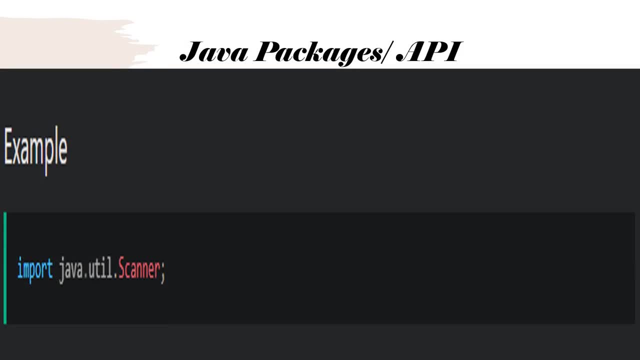 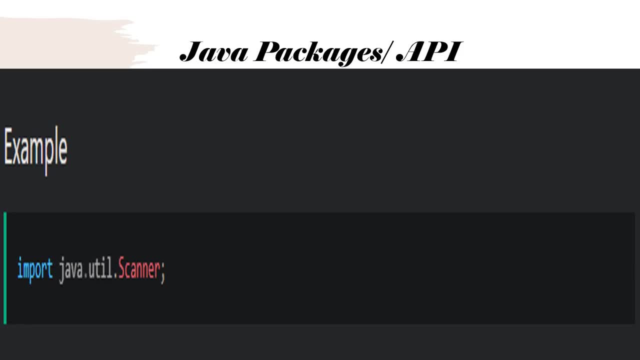 Now if a driver in the agent recipe after the description she did initial is a package, while scanner is a class of the java dot utile package, to use the scanner class, create an object of the class and use any of the available methods found in 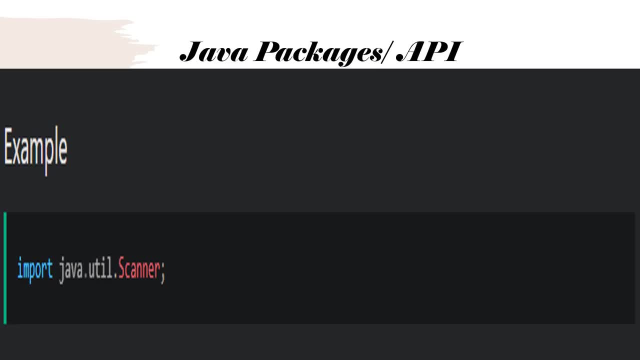 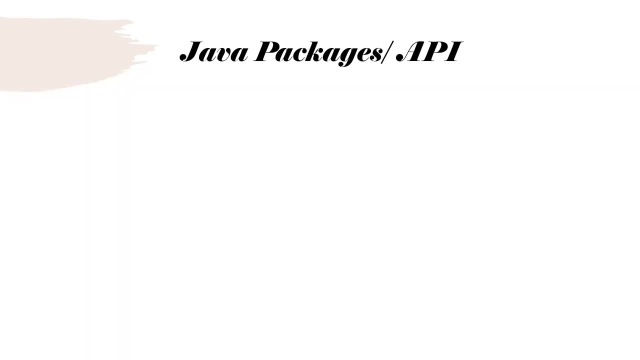 the scanner class documentation. In our example, we will use an extra line method, which is used to read a complete line. 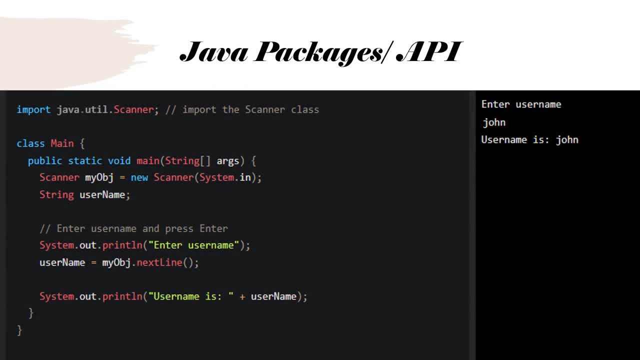 The program is a java code that prompts the user to Enter a user name, reads the input from the keyboard, and prints the entered user name, if you declare an LIA above and click enter and see the J java code.. 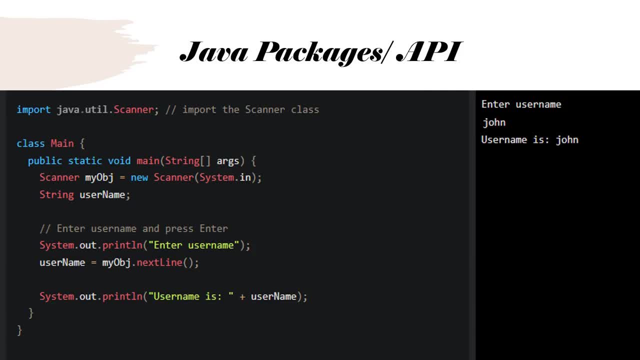 incorrect package name to import it will result in a compile time error this error occurs because the Java compiler can't find the specified package and the required classes and methods can't be found when you declare an import statement in a Java program you are indicating to the Java compiler that you 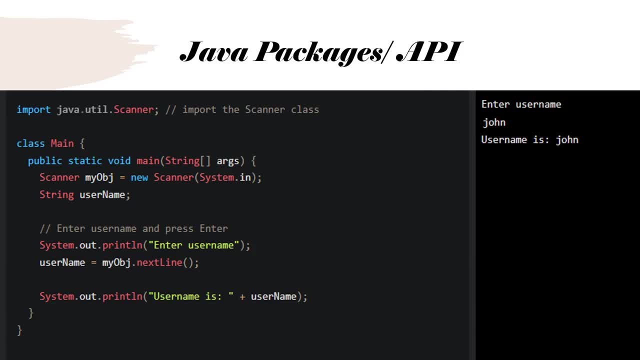 want to use classes or methods from a specific package in your code by importing the Java dot utility scanner package you are able to use the scanner class in your code the purpose of this is to simplify the use of commonly used 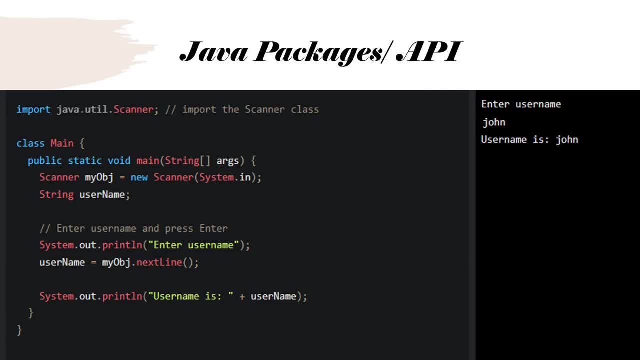 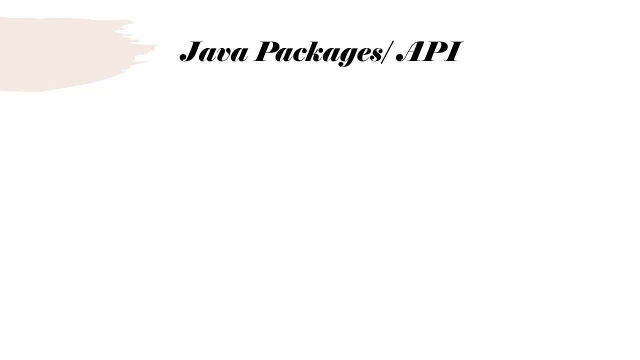 classes and methods so that you don't have to specify the full package name every time you use them this helps to make your code more readable and maintainable when you declare an import statement it's important to ensure that the package you are importing exists and is available in the class path otherwise a compile time error will occur import 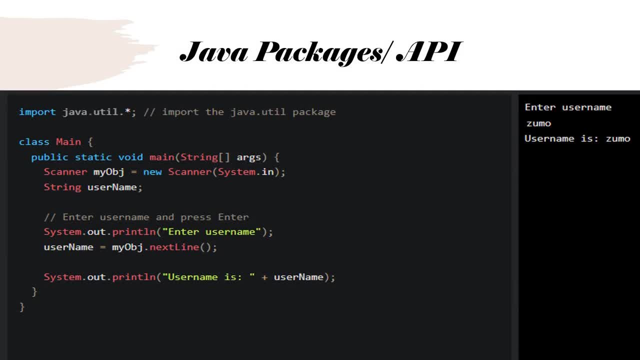 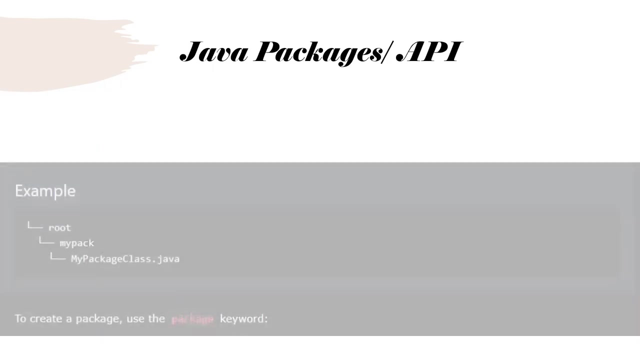 a package there are many packages to choose from in the previous example we use the scanner class from the Java dot util package this package also contains date and time facilities random number generator and other utility classes to import a whole package end the sentence with an asterisk sign the following example will import all the classes in the Java dot util package user-defined packages to create your own package you need to understand that 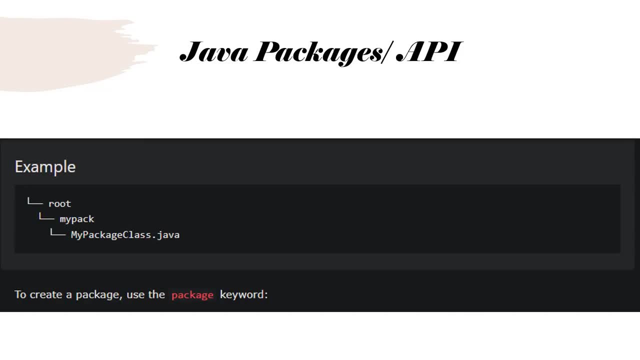 Java uses a file system directory to store them just like folders on your computer to create a package use the package keyword the program is a simple Java code that defines a class named my package class 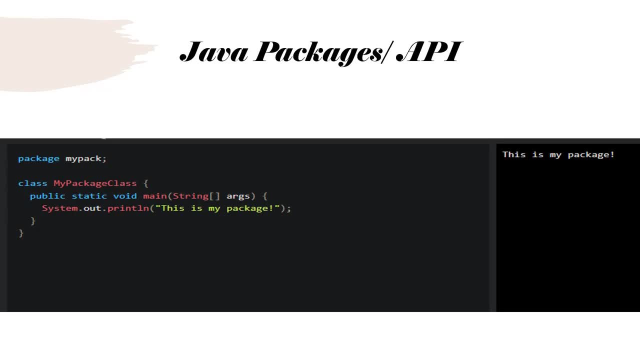 and has a main method that prints the message this is my package dot the significance of the package my pack in the program is that it specifies the specifies a unique namespace for the ClassMyPackage class. This package name ensures that the ClassMyPackage class does not conflict with other classes that may have the same name, but are in a different package. The package name helps to organize your code and makes it easier to manage and maintain. The program flow of the code is as follows. 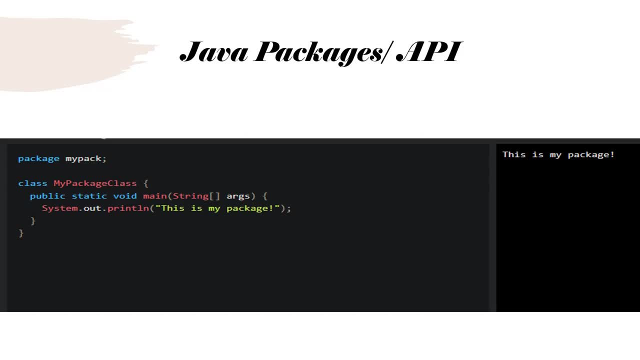 The ClassMyPackage class is declared and defined in the PackageMyPack. The main method is declared inside the ClassMyPackage class. The main method is the entry point of the program and when the program is executed, the main method is automatically called inside the main method. The message, this is my package, is printed to the console. The program terminates after the message is printed. 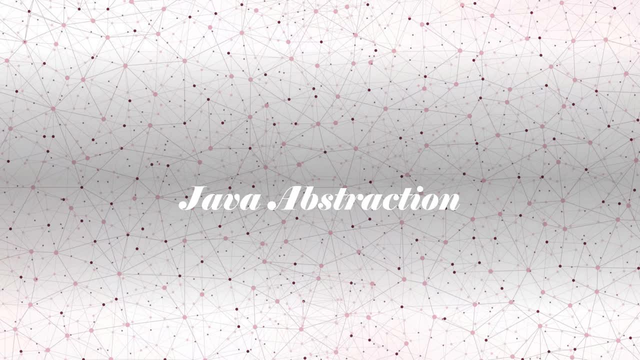 Abstract classes and methods. Data abstraction is the process of hiding certain details and showing only essential information to the user. 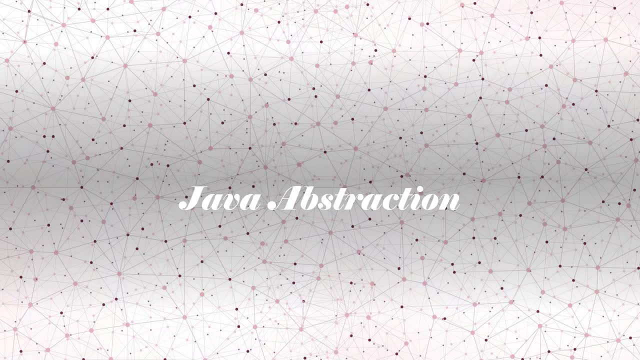 Abstraction can be achieved with either abstract classes 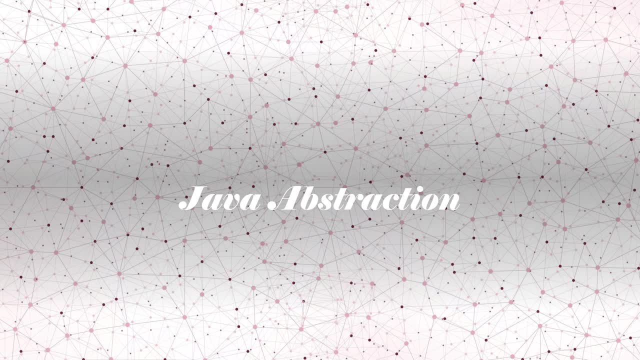 or interfaces, which you will learn more about in the next chapter. The abstract keyword is a non-access modifier used for classes and methods. Abstract class is a restricted class that cannot be used to create objects to access it. It must be inherited from another class. Abstract method can only be used in an abstract class and it does not have a body. 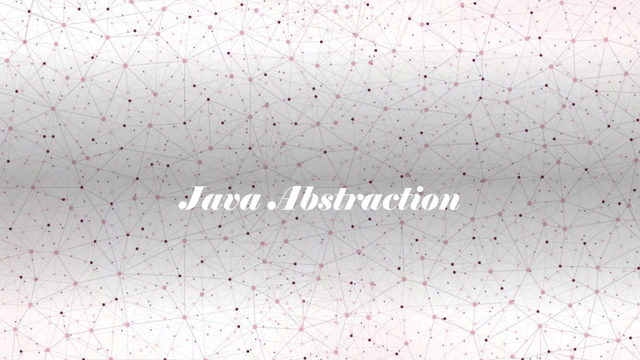 The body is provided by the subclass inherited from . 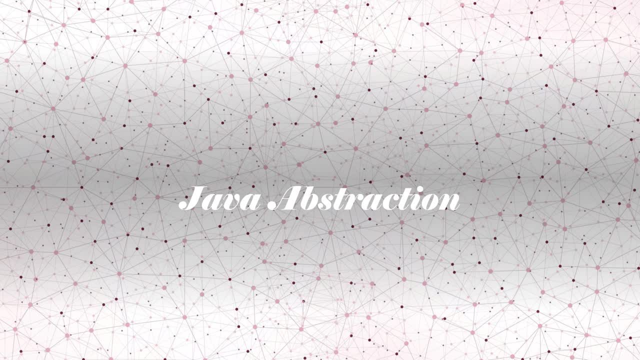 An abstract class can have both abstract and regular methods. 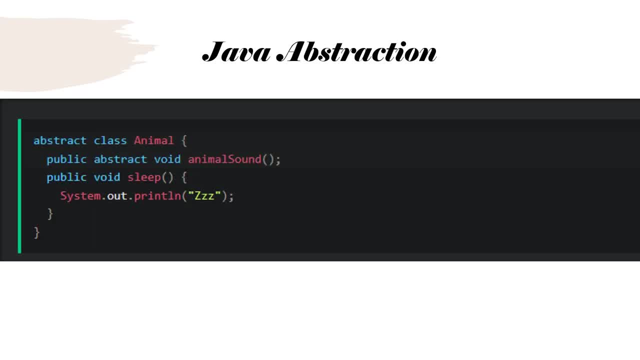 From the example above, it is not possible to create an object of the animal class. 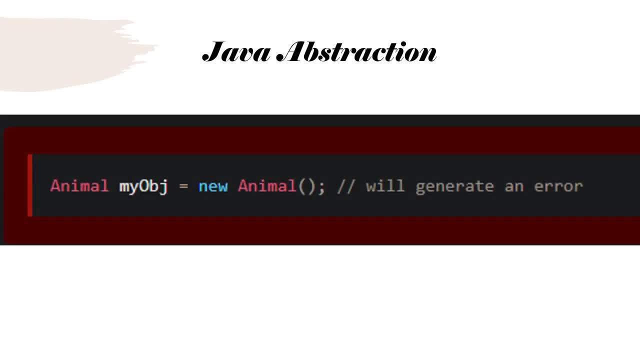 To access the abstract class, it must be inherited from another class. 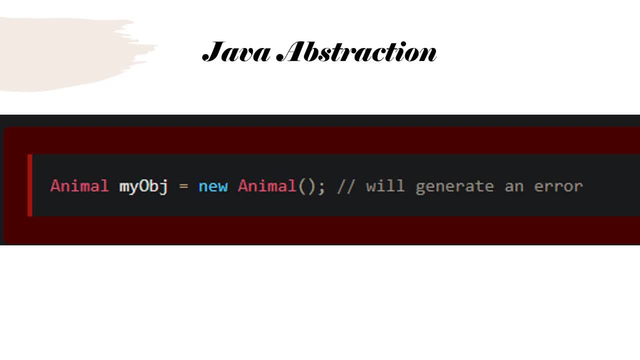 Let's convert the animal class we used in the Polymorphism chapter to an abstract class. 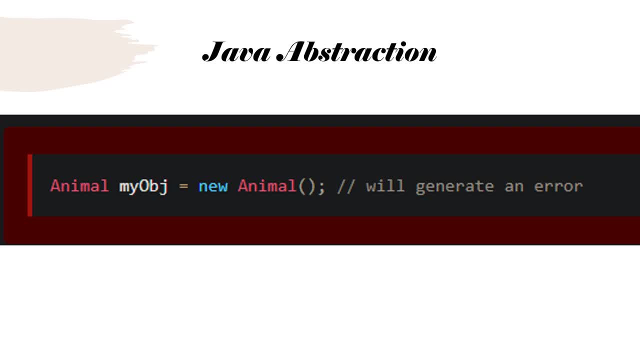 Remember from the inheritance chapter that we use the extends keyword to inherit from a class. 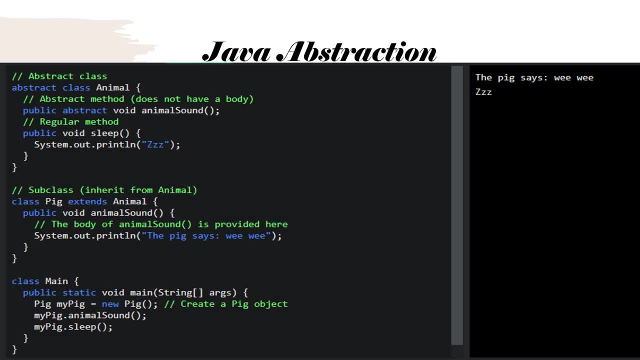 This program is an example of abstraction in Java, where an abstract class animal is defined with an abstract method animal sound and a regular method sleep. A subclass pig is created by extending the animal class and it provides the implementation of the abstract method animal sound. The main class creates an object of the pig class and calls the animal sound and sleep methods, which results in the following output. 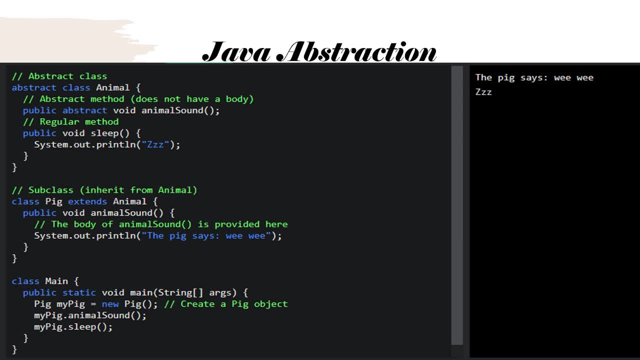 The logic of the program is to demonstrate abstraction in Java, where the abstract class animal defines the general behavior expected from any animal and its subclasses provide the specific implementation for each type of animal. 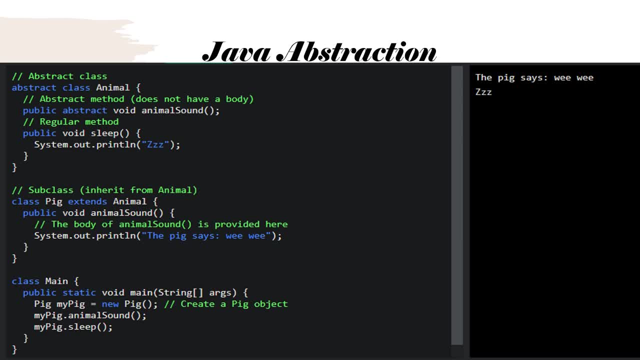 Abstraction in Java is a mechanism of hiding the implementation details from the user and exposing only the necessary information. 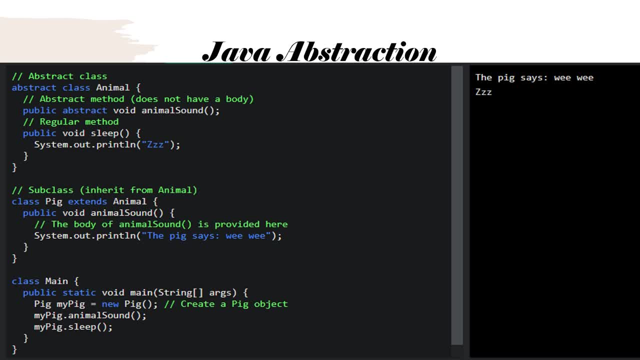 It is used to focus on the essential features of a class without including the background details. 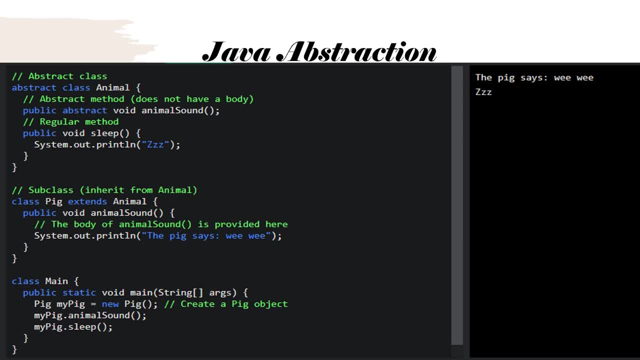 Abstraction is achieved through abstract classes and interfaces in Java. 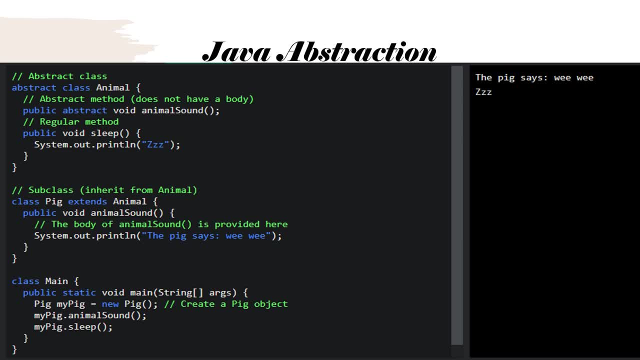 The abstract class can have abstract and non-abstract methods, while an interface can only have abstract methods. 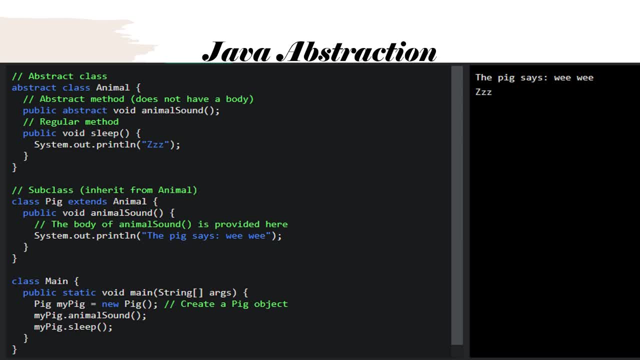 Abstraction helps to reduce complexity and improve modularity in a program. 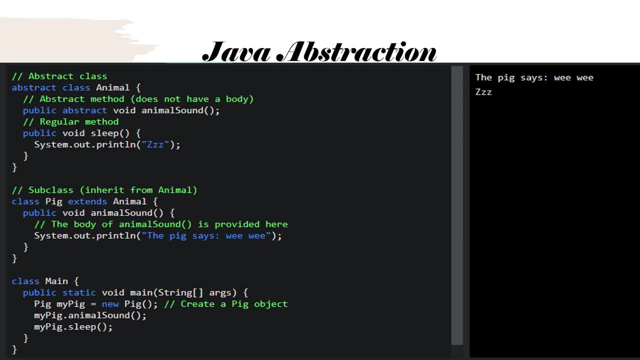 Why and when to use abstract classes and methods to achieve security hides certain details 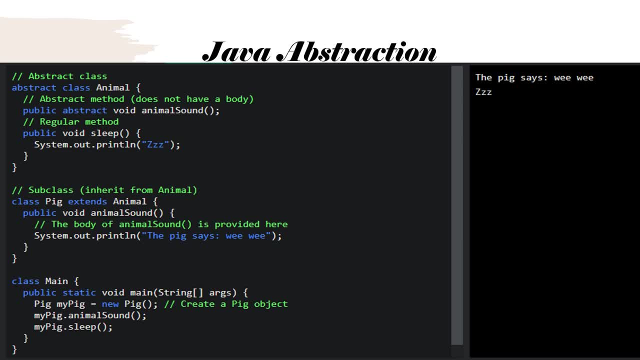 and only show the important details of an object . 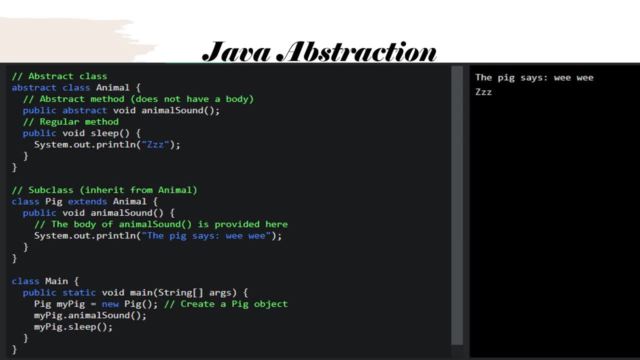 Abstraction can also be achieved with interfaces, which you will learn more about in the next chapter.